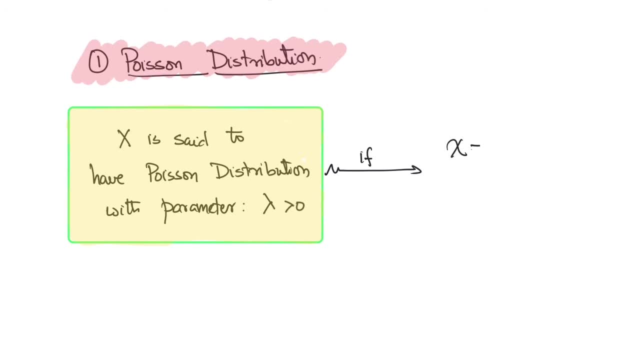 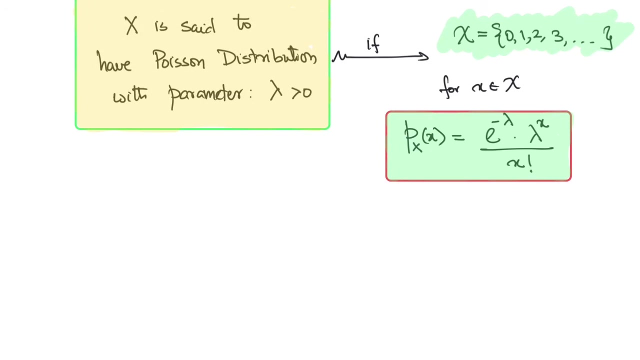 if x takes values in the set all the way up to infinity and the pdf, that is the probability that x equals small x, is going to be defined as e to the minus lambda times lambda to the x divided by x factorial. The first thing we'd want to check is that this is in fact a pdf. 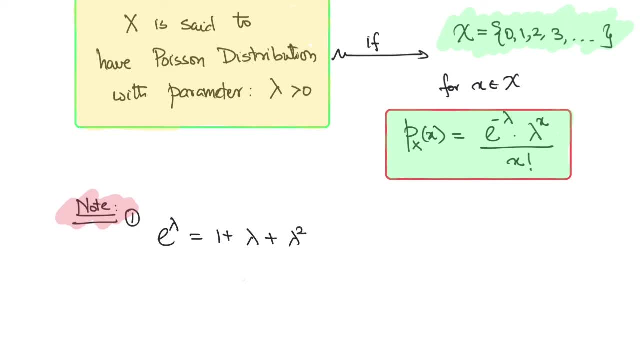 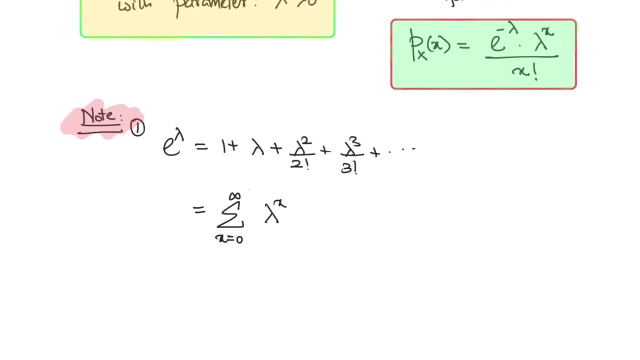 This follows from the fact that e to the lambda has the following infinite series expansion, that is, the sum x going from 0 to infinity of lambda to the x divided by x factorial. So we can write 1 as e to the minus lambda times the infinite sum, so that this simplifies to. 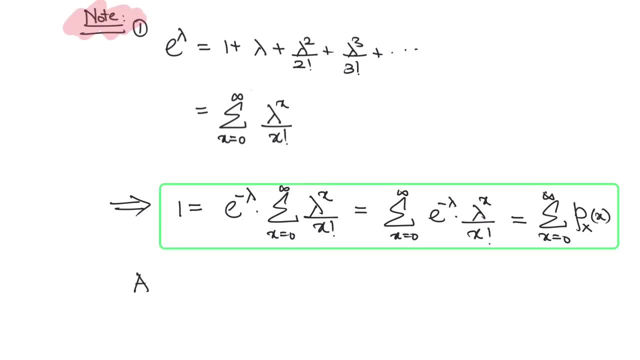 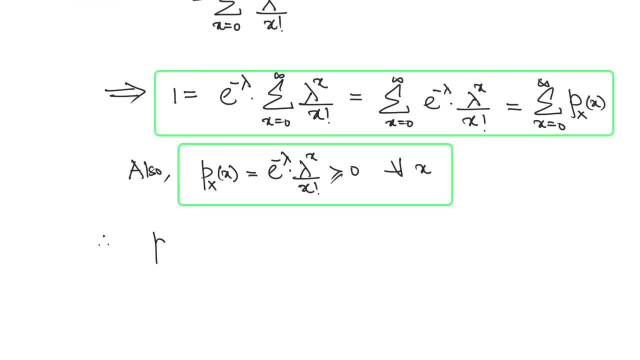 the sum x going from 0 to infinity, of p sub x of x. Also, notice that p sub x of x is greater than equal to 0 for all x and this tells us that p sub x is a legitimate probability mass function. If a random variable x. 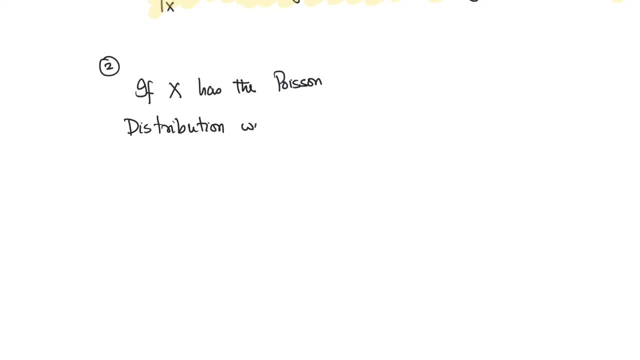 has the Poisson distribution with parameter lambda, then the expected value of x can be calculated to be equal to lambda and the variance of x is going to be also lambda. In this case, the standard deviation is going to be square root of lambda. The Poisson distribution is often used to model phenomena, where we are waiting for events to 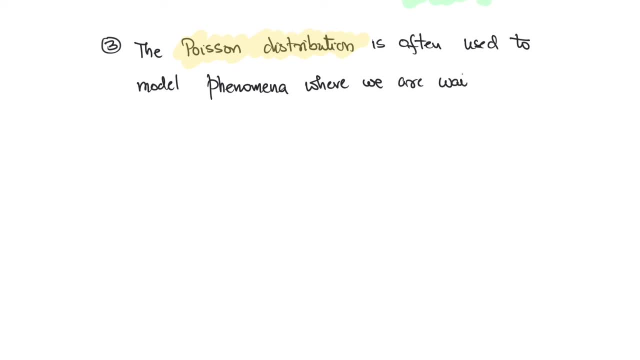 happen and or trying to count the number of events in a given time interval. For example, in the case of a Poisson process, we will use the Poisson distribution to calculate the probability of the number of occurrences in a given time interval. t. We will next talk about the negative binomial distribution. 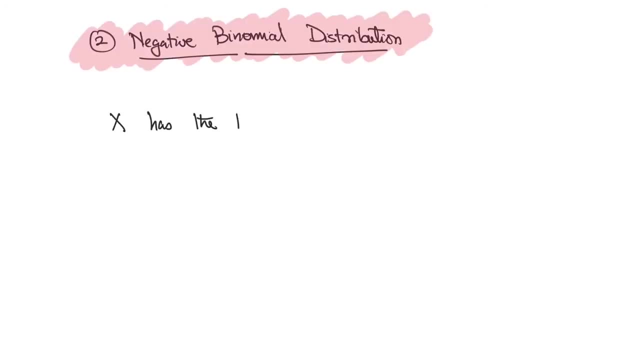 We say that the random variable x has the negative binomial distribution with parameters r and p. If the random variable takes values in the set 0,, 1,, 2,, 3, all the way up to infinity, and if, for any x inside script x, the probability mass function is defined as follows: 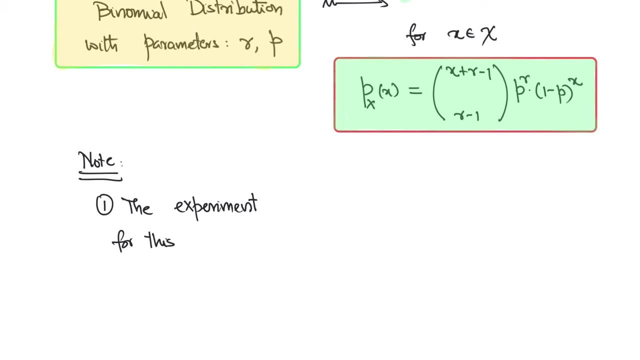 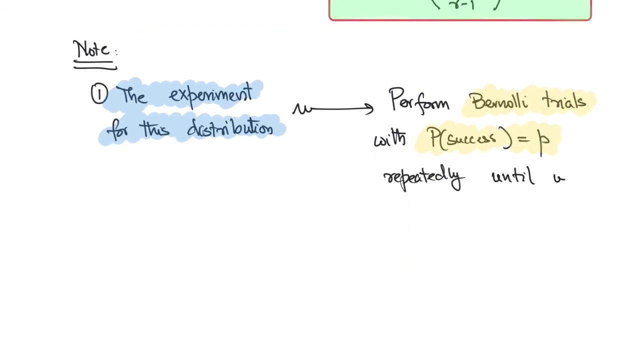 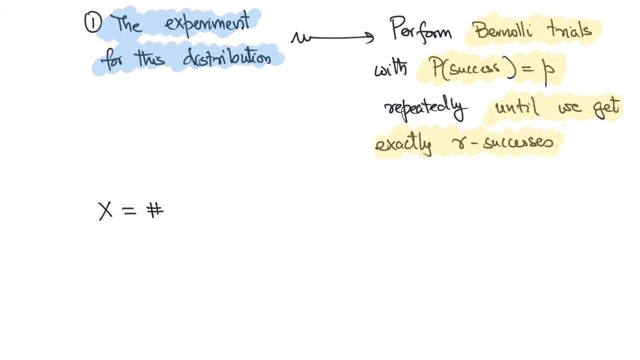 The negative binomial distribution corresponds to the following experiment, where we perform Bernoulli trials with the probability of a success. These are independent Bernoulli trials- repeatedly until we get exactly our successes. The random variable x will then be defined as the number of failures that precede the rth success, In this case the probability. 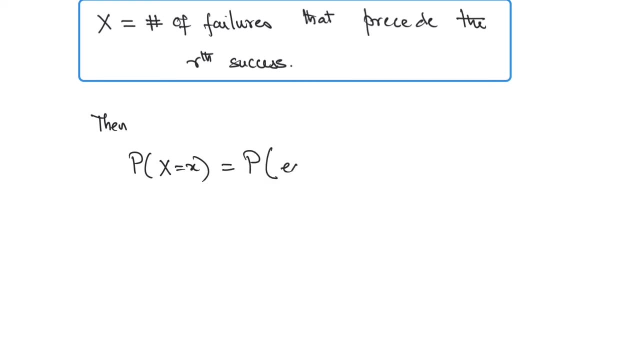 that x equals x is going to be the probability of exactly x failures before the rth success. The total number of ways we can have exactly x failures before the rth success corresponds to the counting problem of choosing x spots in x plus r minus 1 possible places. 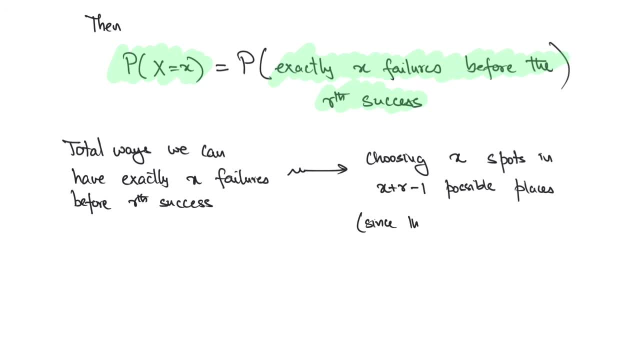 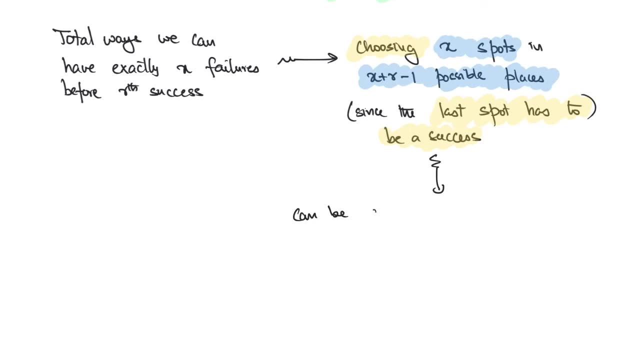 This is the case because the last spot has a success and hence is fixed. This can be done in x plus r minus 1 choose x ways, which is the same as x plus r minus 1 choose r minus 1 ways. So, putting this back together, we: 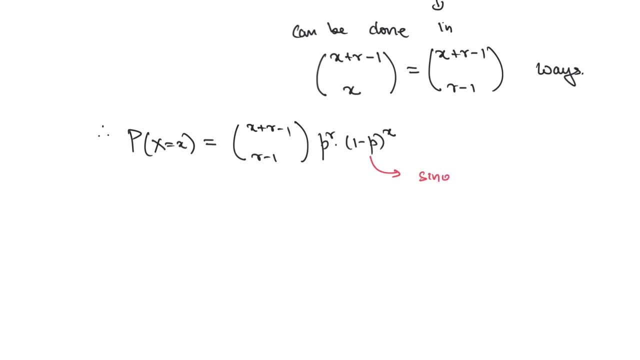 notice that the probability of x equals x is going to be given by the following formula, which is exactly the PMF of the negative binomial distribution. If x has the negative binomial distribution with parameters r and p, the expected value of x is going to. 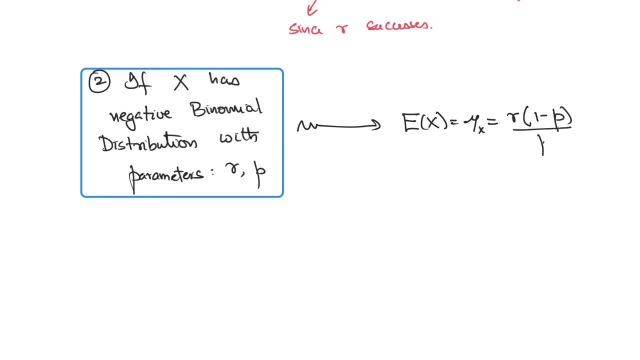 be r times 1 minus p divided by p, and the variance of x can be calculated to be r times 1 minus p divided by p squared. This distribution is called a negative binomial distribution because x plus r minus 1. choose x can be written as minus 1. choose x minus 1. minus 1 minus 1. 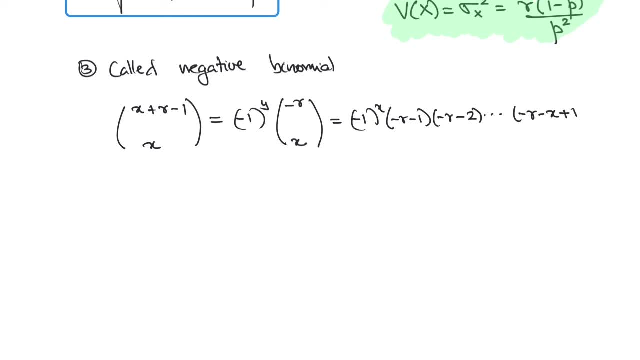 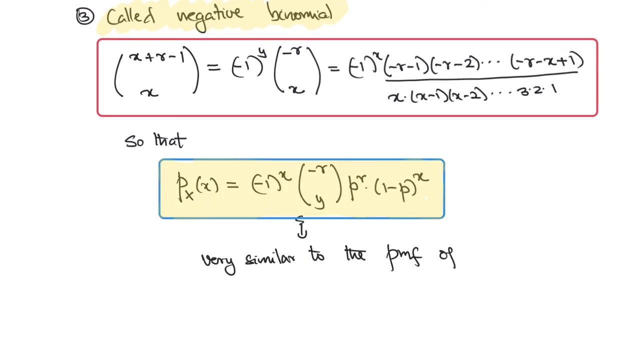 to the y times minus r, choose x. So, putting this into the distribution function, we notice that p of x is going to be equal to minus 1 to the x times minus r, choose x. There is a typo in the video: times p to the r, times 1 minus p to the x. This is very similar to: 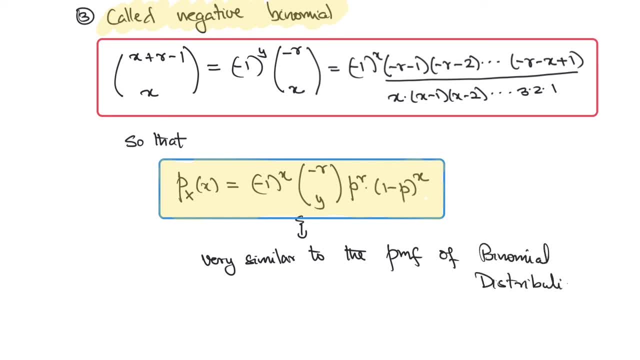 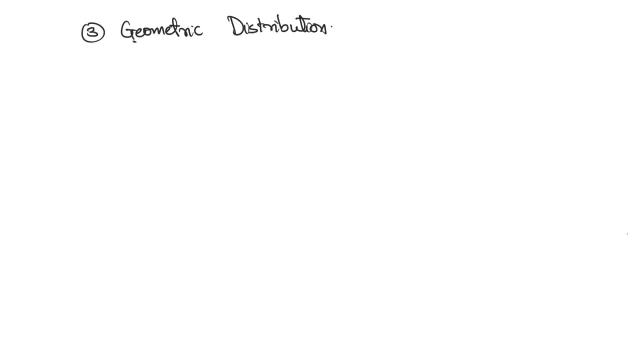 the PMF of the binomial distribution, We move on to our final distribution for today, which is going to be the geometric distribution. We will say that x has a geometric distribution with parameter p if x takes values in the set 1,, 2,, 3,, all the way up to infinity. Note that, unlike the previous two distributions, 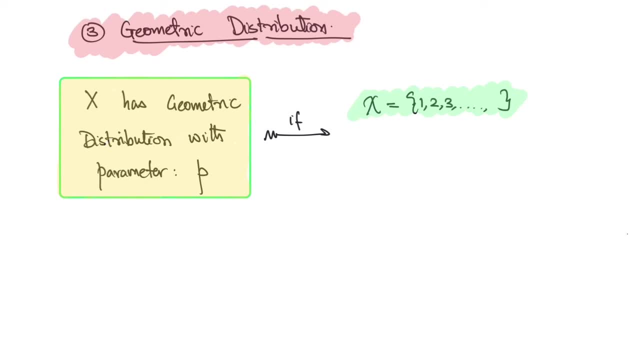 zero is not in the set of values for x. here The PMF for this distribution is given by p sub x of p. This is the p of x of the binomial distribution. So if x is equal to 1,, 1 minus. 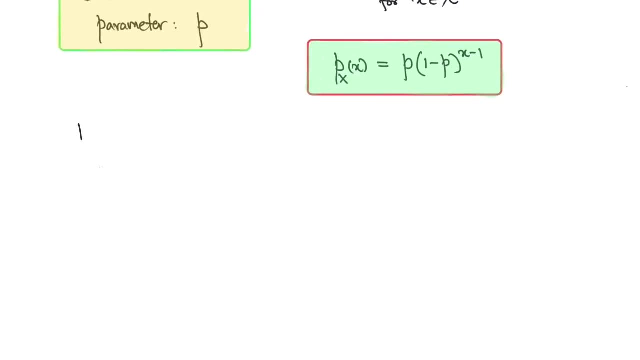 of x equals p times 1 minus p to the x, uh to the power, x minus 1.. the geometric distribution is a special case of the negative binomial probability mass function. when r equals 1 and we're looking at values of x equals 1, 2, 3 up to infinity. 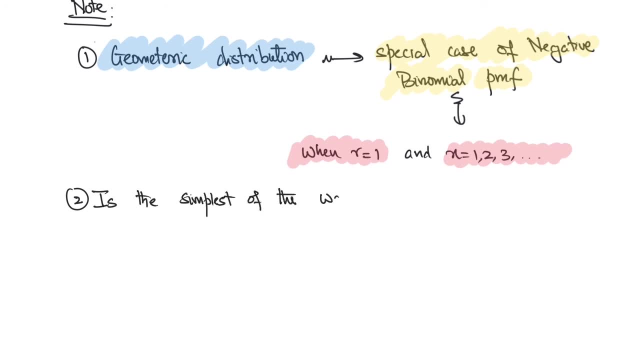 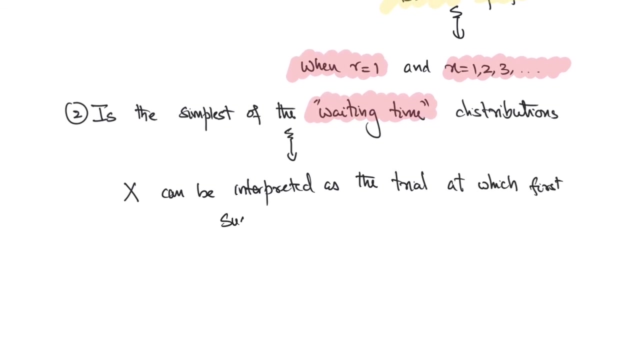 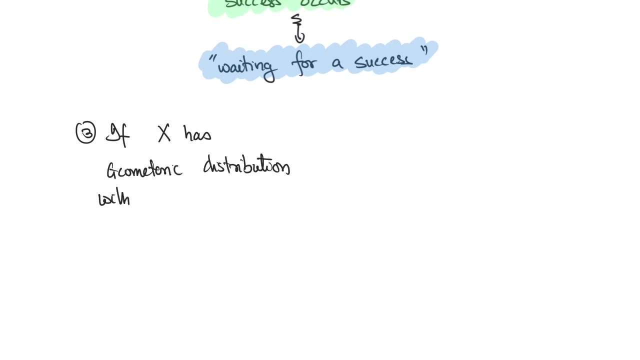 it is also one of the simplest waiting time distributions where we can interpret x as counting the trial at which the first success occurs, which would be me same as saying that we're waiting for a success. if x has the geometric distribution with the success parameter p, we can calculate the expected value of x to be equal to 1 over p and the variance of x. 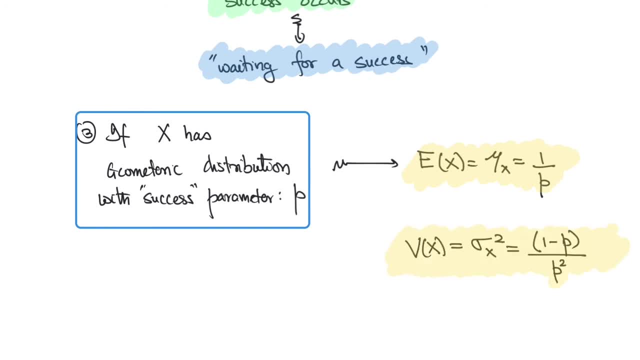 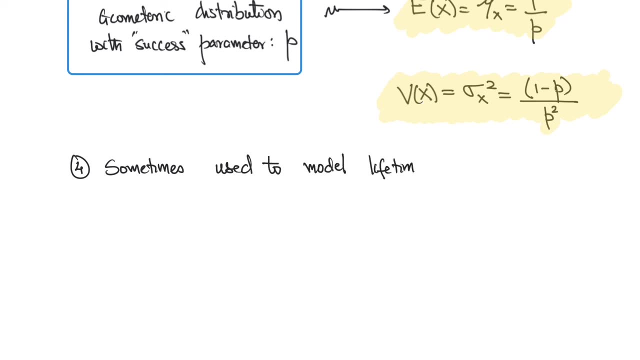 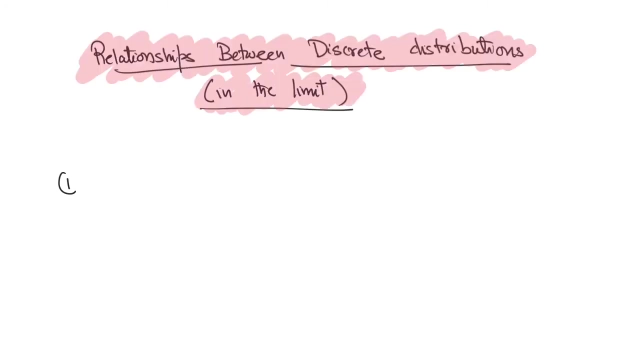 can be calculated as 1 minus p divided by p squared. sometimes one can use the geometric distribution to model the lifetime or the time until failure of components. we will calculate the final result and wrap up this video working out some relationships between discrete distributions that happen in the limit. uh, we'll begin with the binomial hypotrometric. 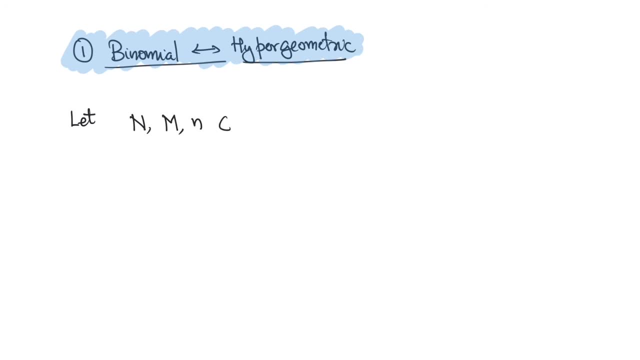 relationship. let a capital n, capital m and small n be natural numbers and let p equals m over n, then the binomial uh, pmf, uh, denoted by b, i, n, X, n, cubed p, where n is the samples size and p is the popular probability of success. 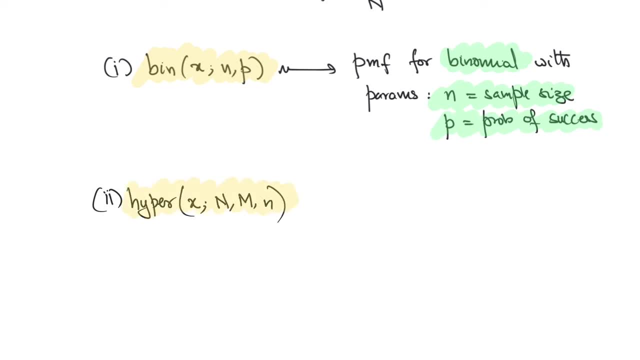 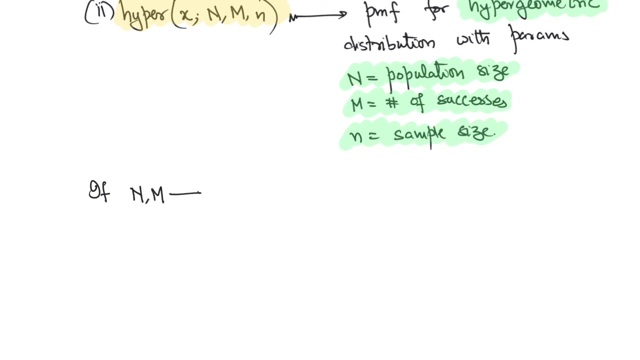 similarly, the hyper geometric PMF is denoted by hyper and it has parameters: capital N, which is the population size, capital M, which is the number of successes on the population, and n is the sample size that we are going to sample from the population. in this setting, if capital N and M both go to 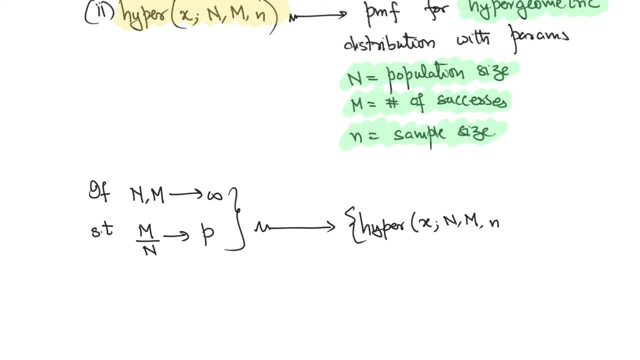 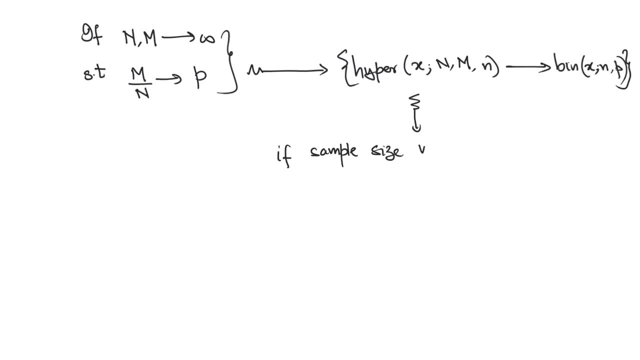 infinity, such that the quotient numero n converges to p, we will have the hyper geometric PMF to converge towards the binomial PMF with parameters X and NP. That is to say that if the sample size n is small compared to the population size, we 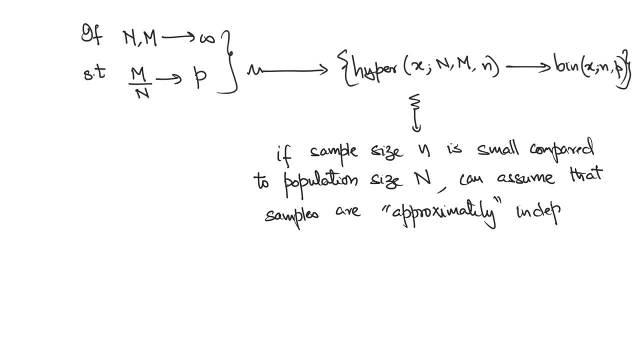 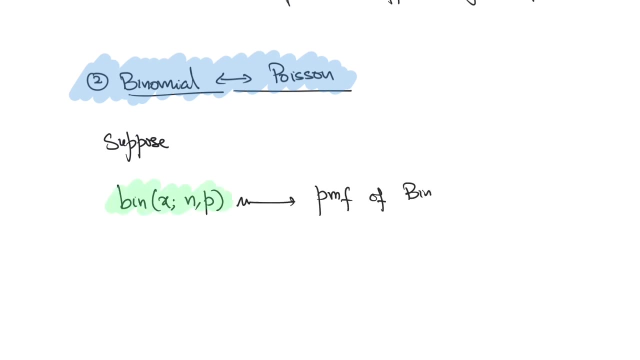 can assume that the samples are approximately independently constructed. The binomial Poisson connection will be next: Suppose b, i, n, x, n, p is the binomial probability mass function with parameters n- the sample size, and p- the probability of a success, and p o poiss, that is, p o i s x comma lambda. 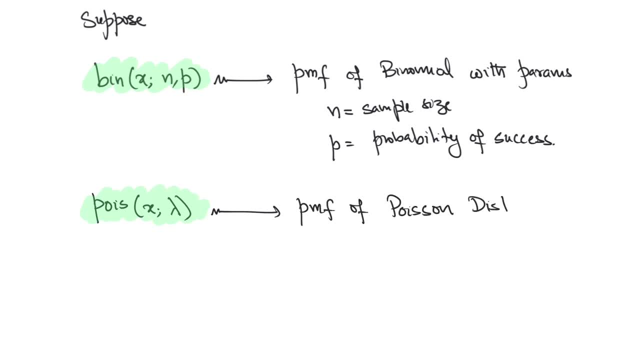 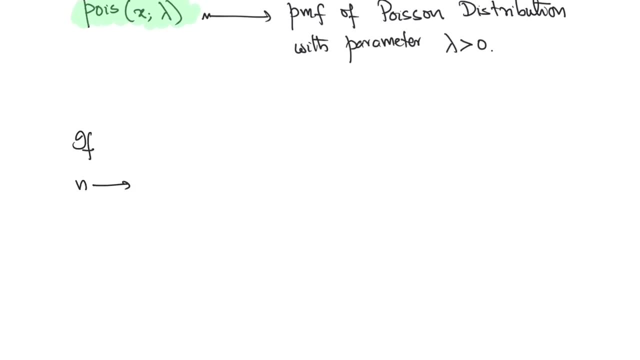 is the probability mass function of the Poisson distribution with parameter lambda. In this setting, if we have n going to infinity and p going to zero, such that the product n times p converges to lambda, we will have the binomial PMF to. 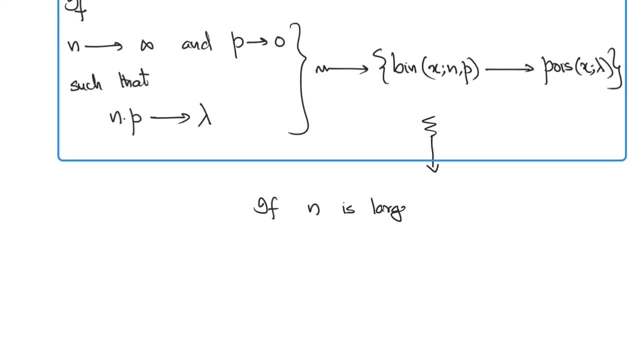 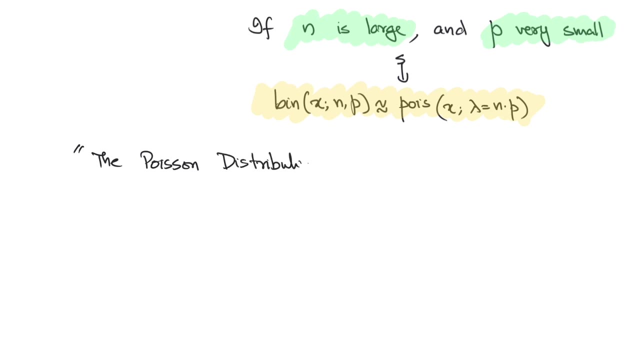 converge to the Poisson PMF. This is the same as saying that if n is large and p is very small, the binomial PMF is going to be very similar to the Poisson PMF. Another way of saying this is that the Poisson distribution